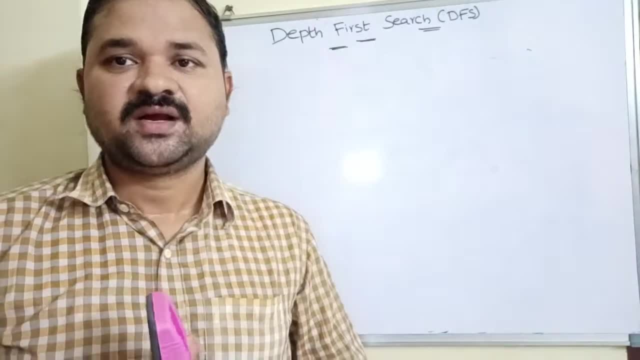 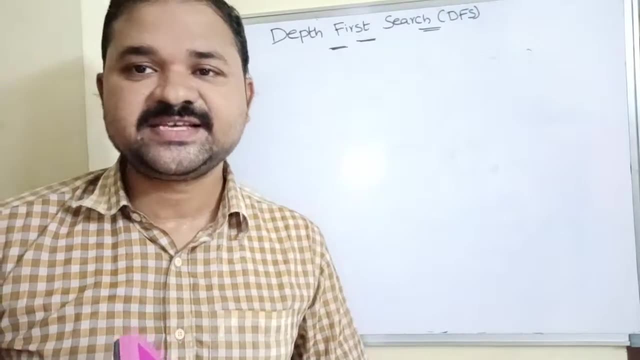 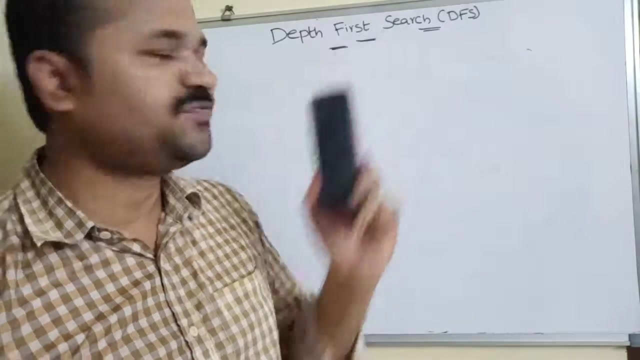 Now let's see about Depth to Facet. Depth to Facet is a graph traversal technique. Graph traversing means visiting the vertices or the nodes of the graph. We can traverse the graph in two ways. The first way is Depth to Facet and the second way is Depth to Facet. 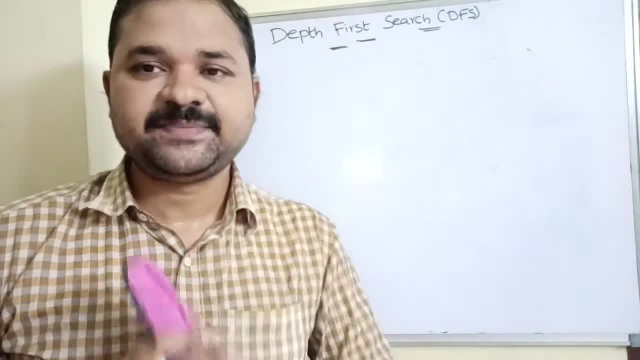 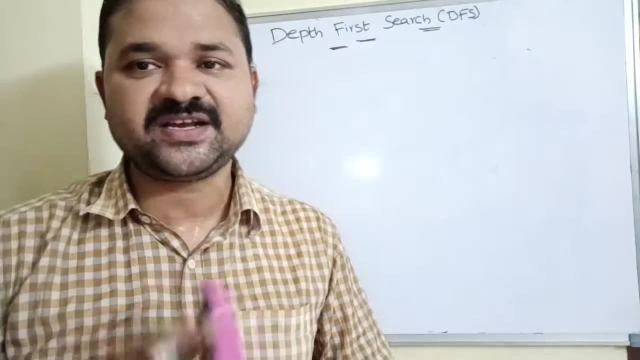 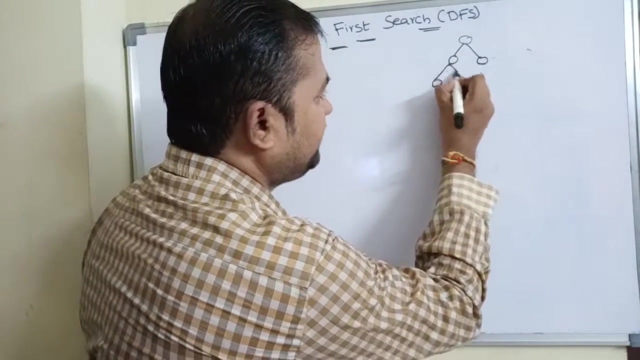 In this video we are going to discuss about Depth to Facet. Depth to Facet means visit all the vertices up to the deepest level and continue so on. So let we have a graph like this. Let us assume that this is the starting vertex. 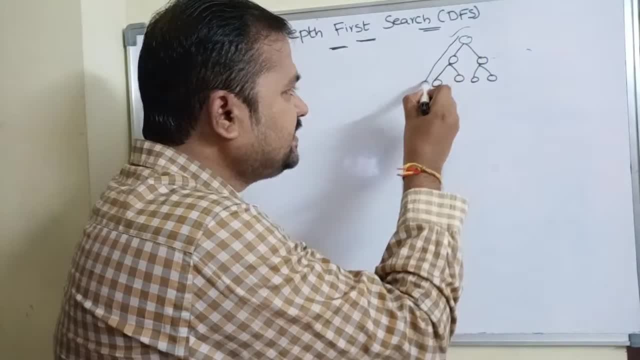 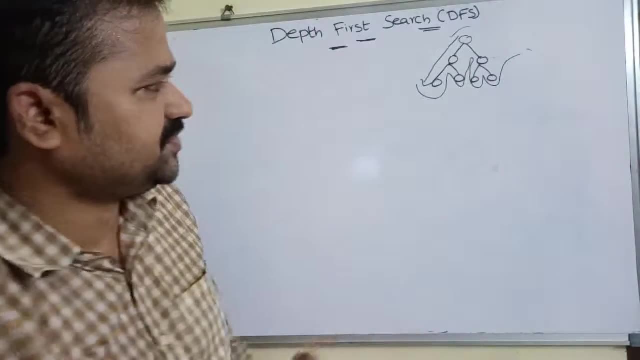 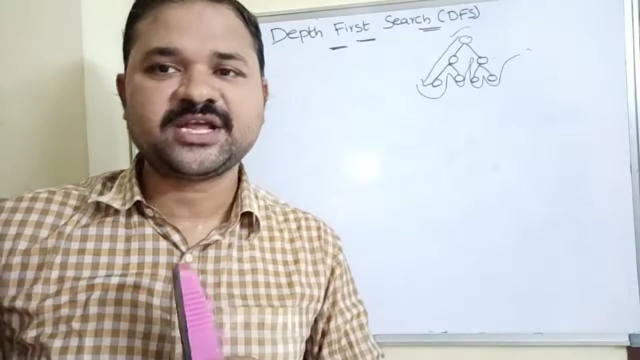 So we have to visit all the vertices till the deepest level and we have to traverse like this to perform some backtracking and pushing operations and visit all the nodes. so here the basic principle is: let us start from a starting vertex and examine and visit all the nodes till we get the deepest. 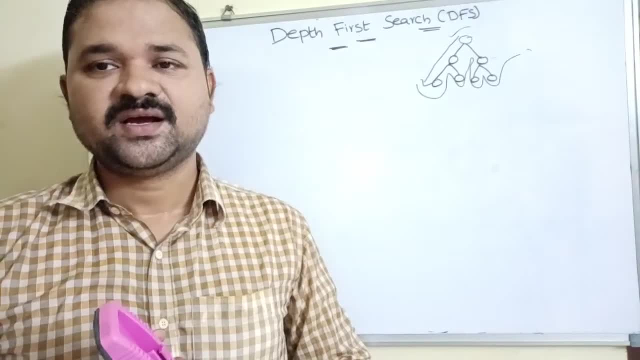 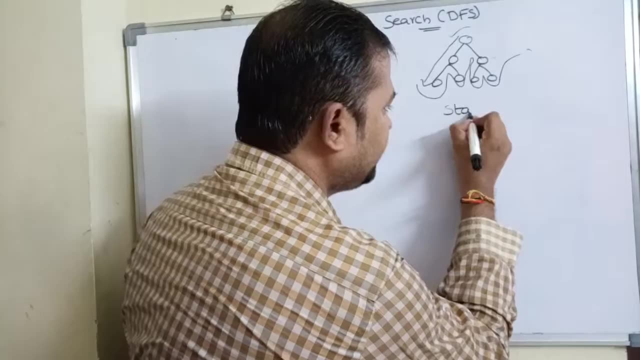 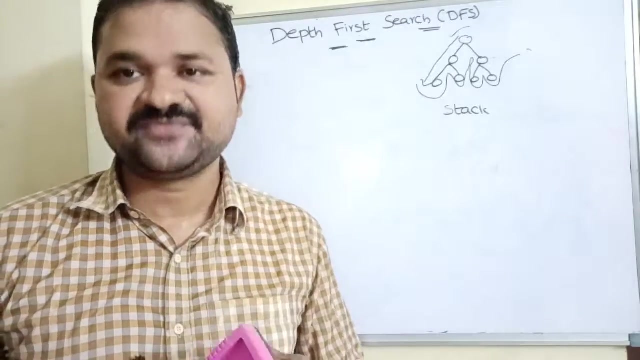 level and go to the previous levels like this. okay, dfs uses a data structure called stack for its implementation, whereas we know that bfs uses q for its implementation, whereas dfs uses stack for its for its implementation. now let's see the algorithm for the dfs depth of assets and then 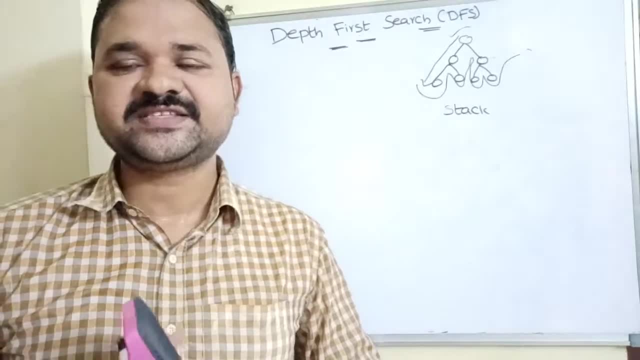 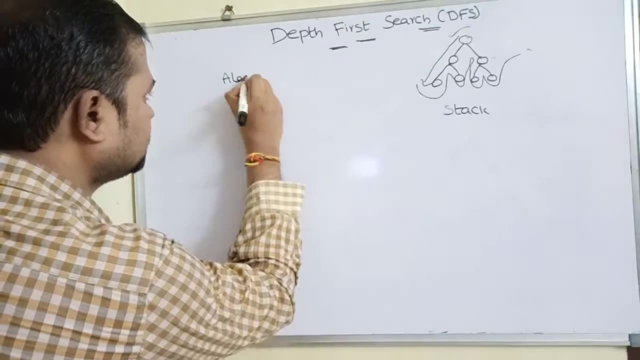 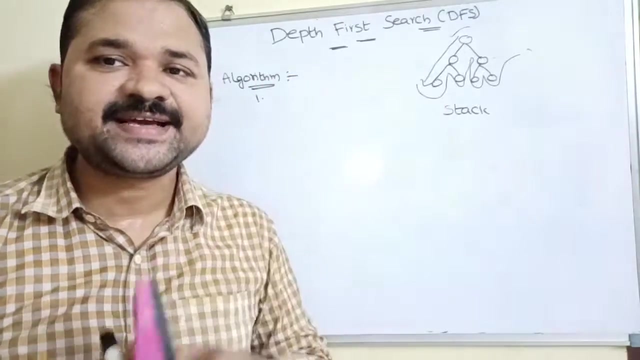 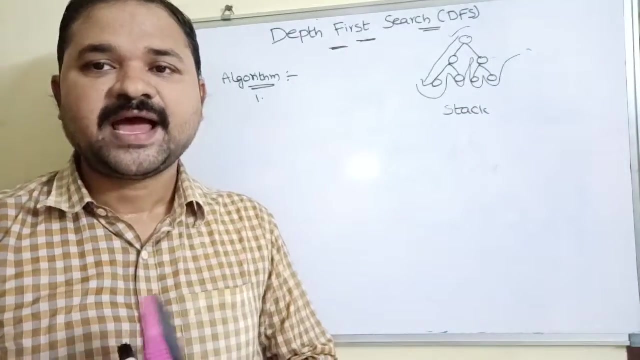 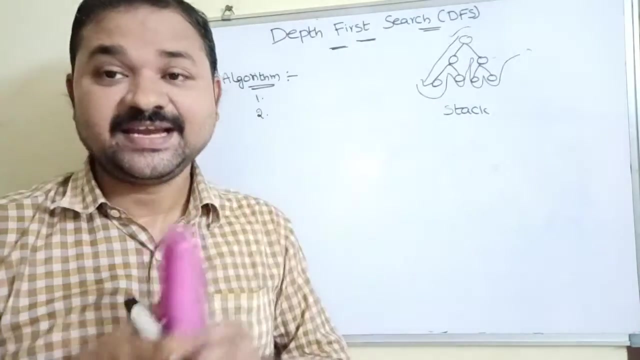 with the help of an example, we will demonstrate dfs algorithm in detail. so let's see the first step here: dfs algorithm. so let's see the first step. take any vertex as the starting vertex and insert it onto the top of the stack and make the status as visited okay. second step: while the stack is not empty, we have to perform. 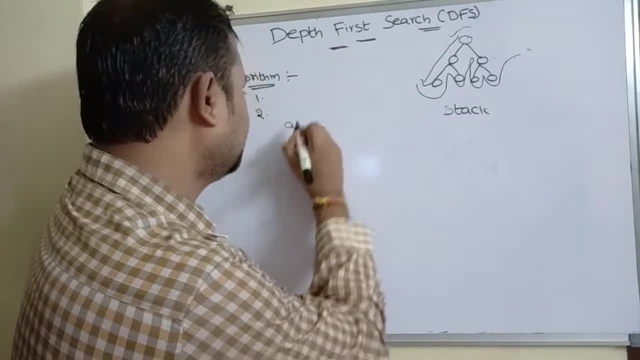 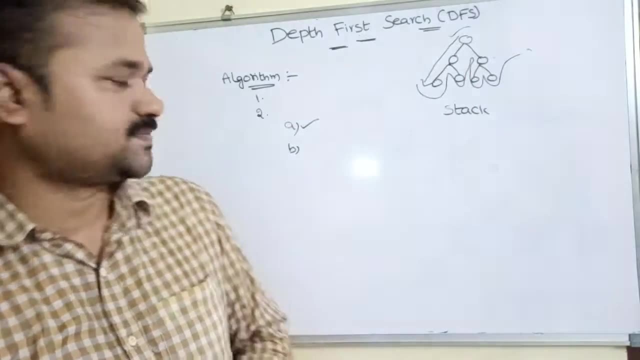 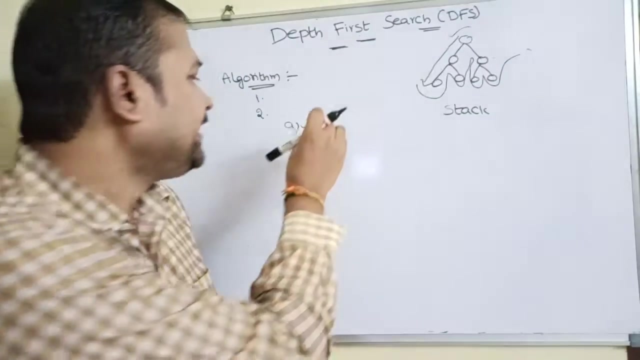 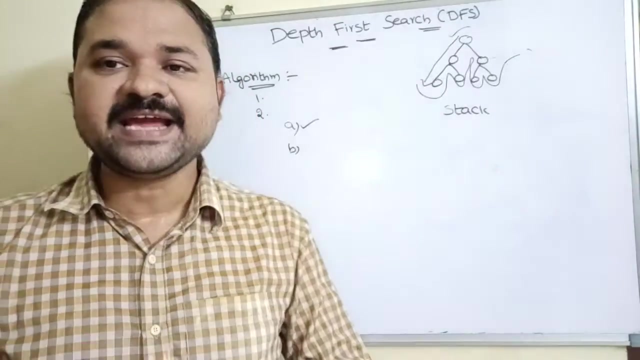 two steps: first one, second one. so let's see the first one: select any unvisited adjacent vertex of the corresponding vertex. that is nothing but the vertex which is at the top of the stack, and insert that into the stack. so what we are doing here: select any unvisited adjacent vertex of the corresponding vertex. 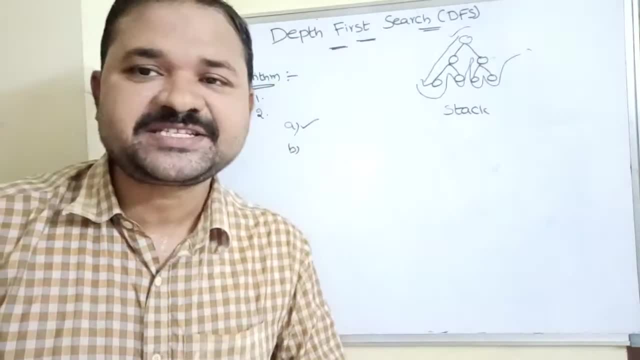 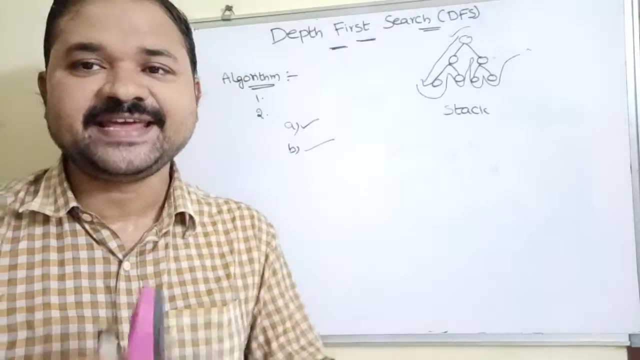 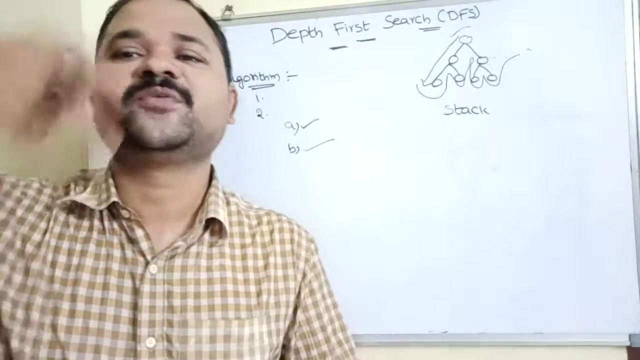 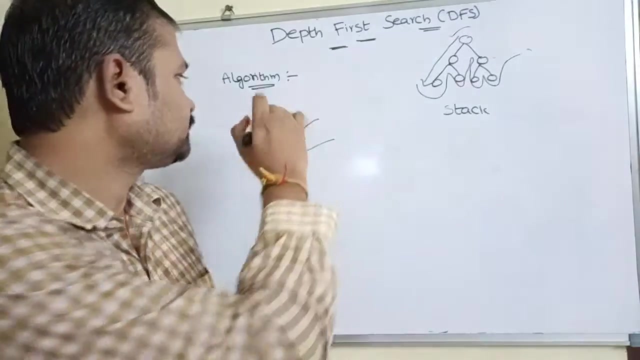 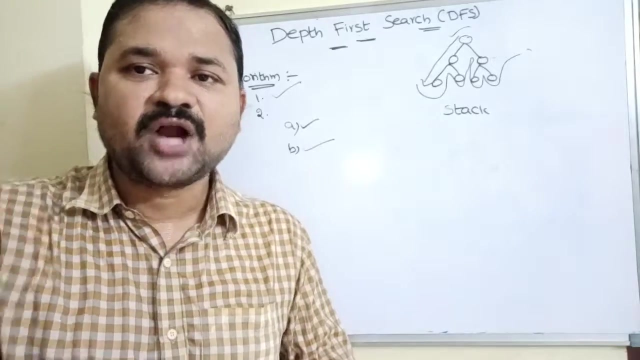 and push it onto the stack and make the status as visited. next step: if there is no unvisited vertex, then perform backtracking and then pop an element from the stack. so simply, how many steps we have here. we have two steps. what is the first step? select any vertex as the starting vertex and push it on to the top of the stack. 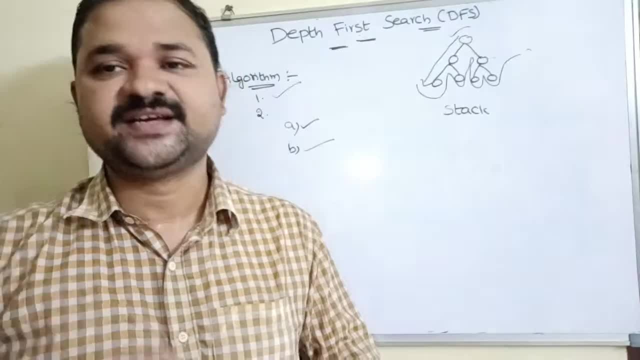 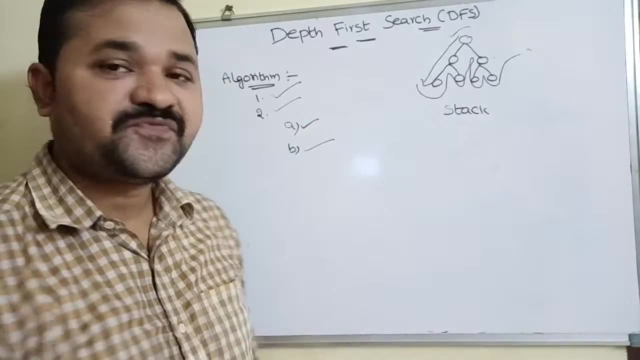 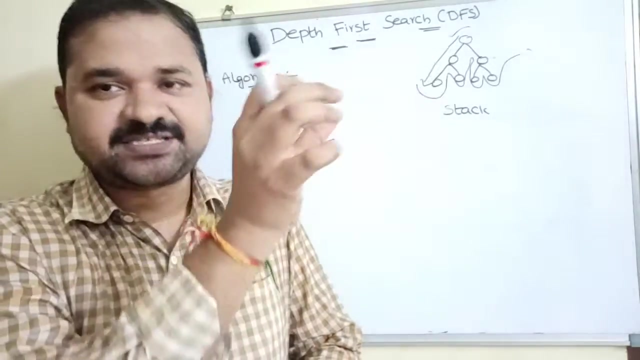 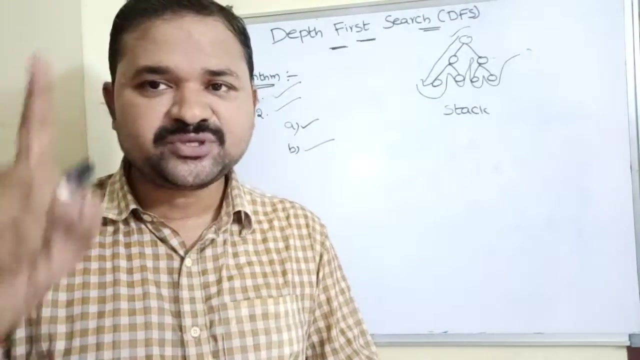 and make their status as visited. so make the status of that starting vertex as visited, okay. next step: while the stack is not empty, then we have to perform two activities. first activity: that vertex, that top vertex, may contain any number of adjacent vertices, out of all which we need to select one unvisited adjacent. 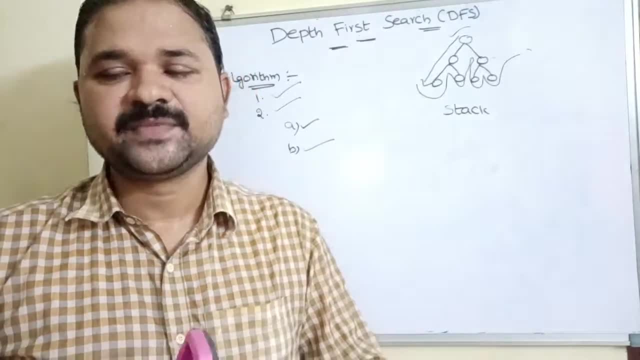 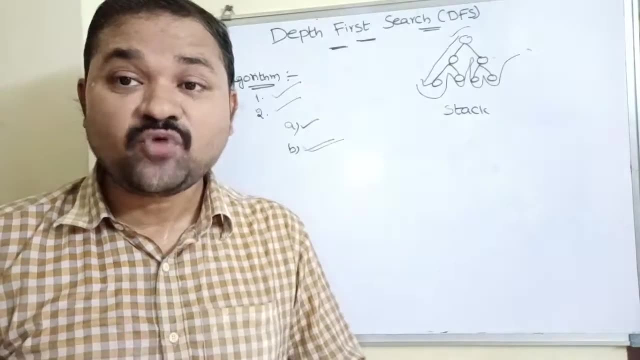 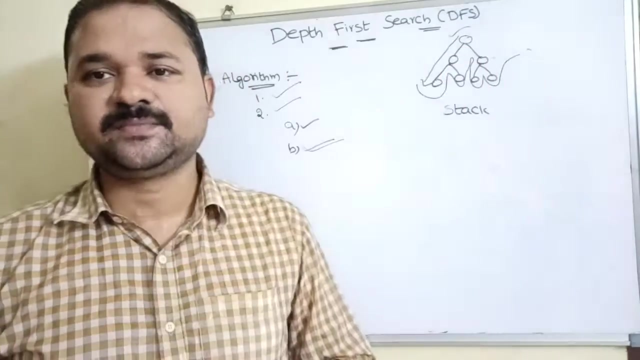 vertex and push it on to the top of the stack and make that vertex status as visited and be with. if the there is no vertex to visit, then perform the backtracking. that means move to its previous level and then pop the stack. pop the stack. so this is the algorithm. 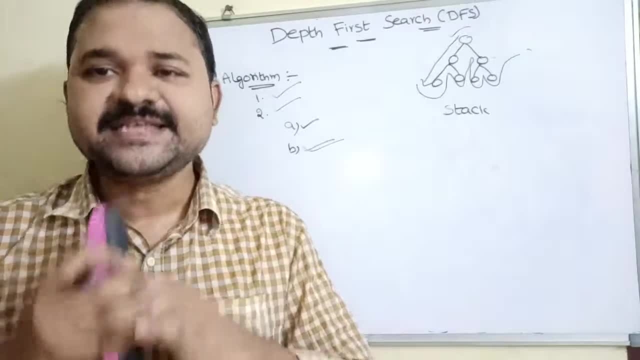 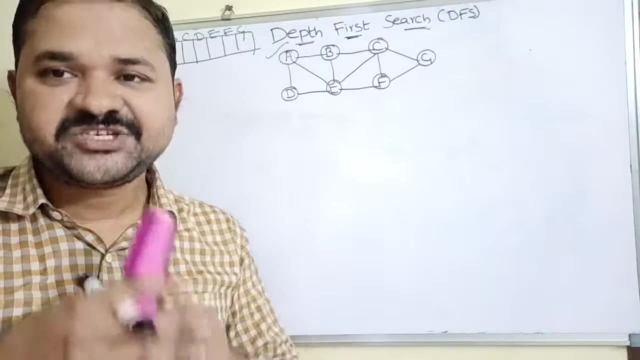 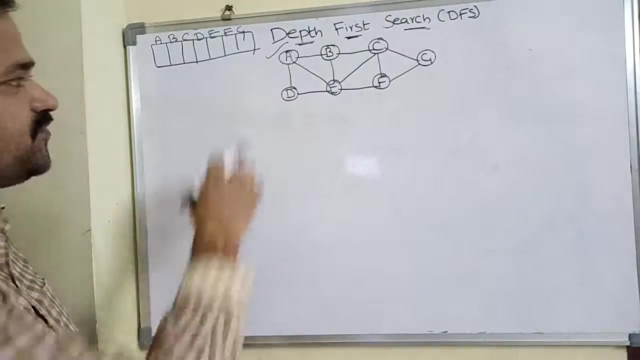 now with the help of this algorithm. let us see an example now. let us solve this problem with the help of DFS algorithm. initially, we have to select one of the vertex as starting vertex. let A be the starting vertex. so we have to insert A on to the top of the stack and make A status as visited. 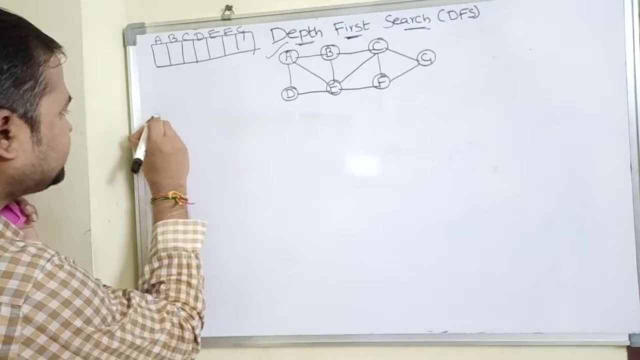 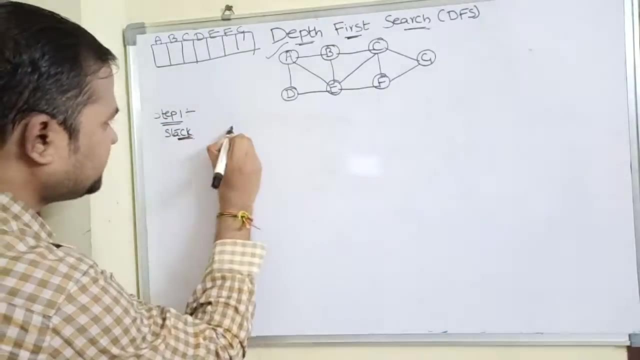 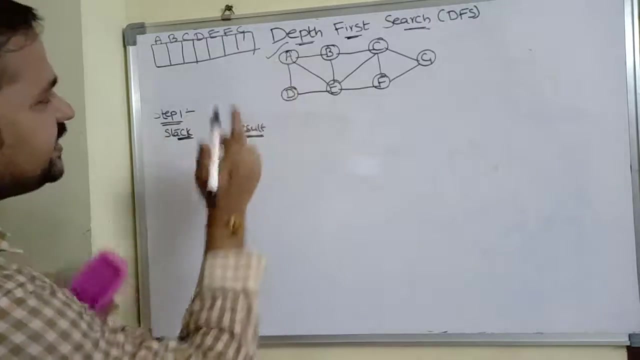 okay, so we have to do these activities. let us write step one here. so step one here. we have stack as well as result. so result specifies that the order in which we are visiting the vertices are nodes. so initially we are assuming that A as the starting vertex, so push A on to the top of the stack. 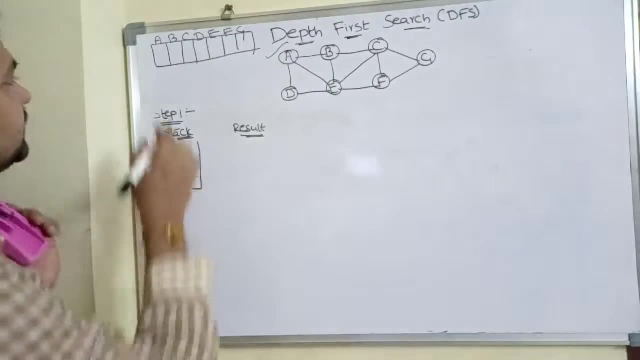 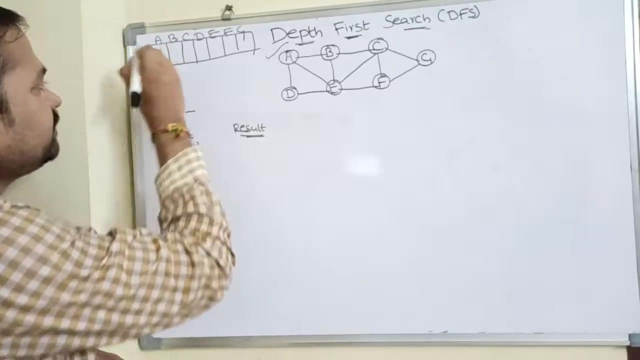 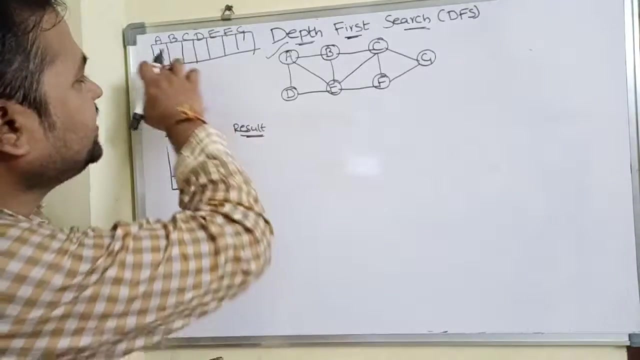 so A is pushing. this is nothing but a visited matrix. so initially A is visited. so we have to make each status as one. so one specifies that the vertex is visited. various zero specifies that the vertex is not visited. initially all the elements are filled up with the zeros. so whenever 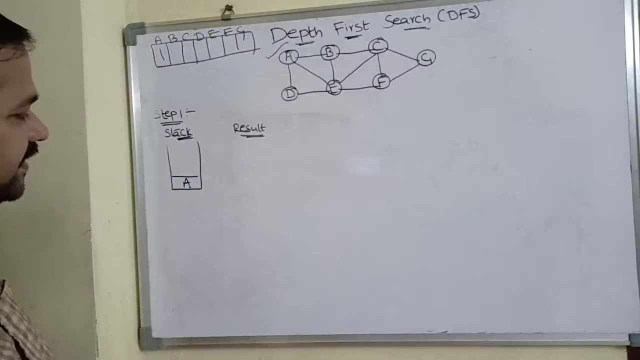 we visited the any vertex, then we have to insert one there. okay, so A is visited, so the output is A. okay, let us write state one to the left and a slash. So if the object is visited, Celsius, like this in this particular case, this is the output of vertex A. Please note that always missed an handicapped trajectory Coach, always eliminated or missing when seeded any item for any cheque. 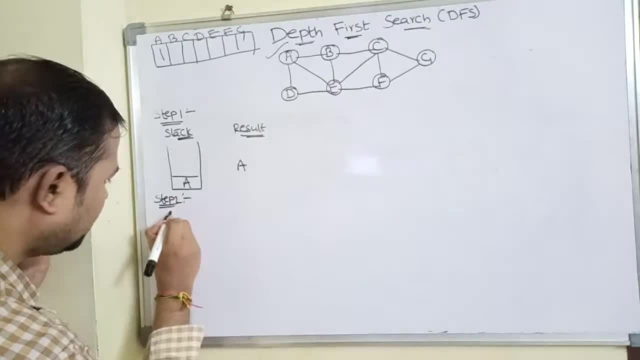 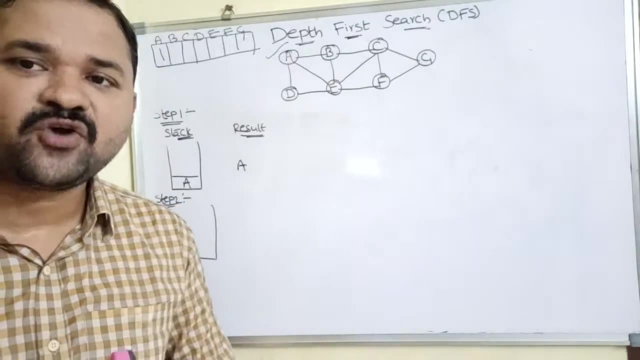 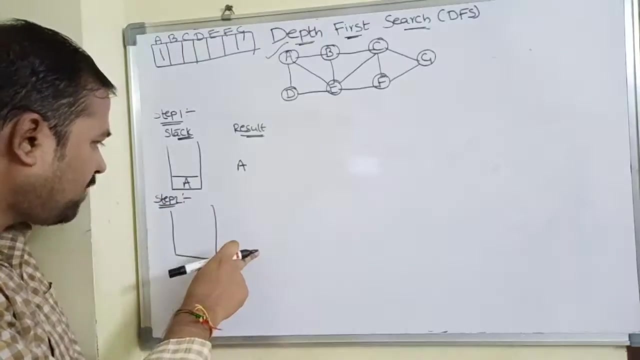 step 2.. So what is step 2?? In step 2, we have two operations. While the stack is not empty, then we have to select one of the unvisited adjacent vertex which is available in top of the stack. So we have to. first we need to select the adjacent vertices of A, out of which 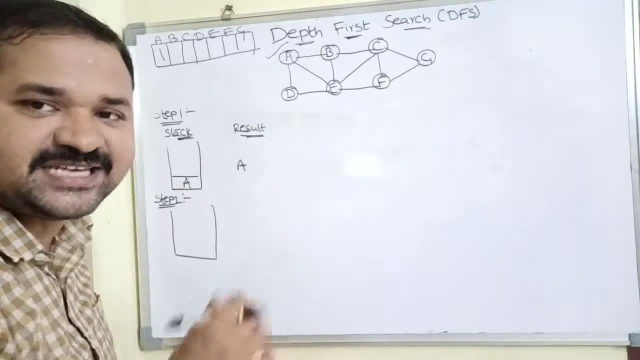 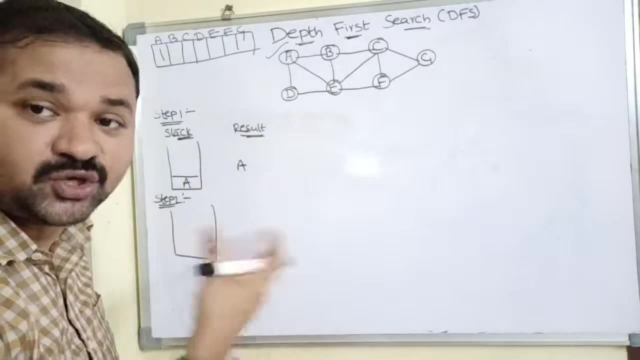 we have to select one of the unvisited adjacent vertex and push it onto the top of the stack and make the status as visited Suppose. if there is no need, no node to visit, then we have to perform the backtracking as well as perform the pop operation. 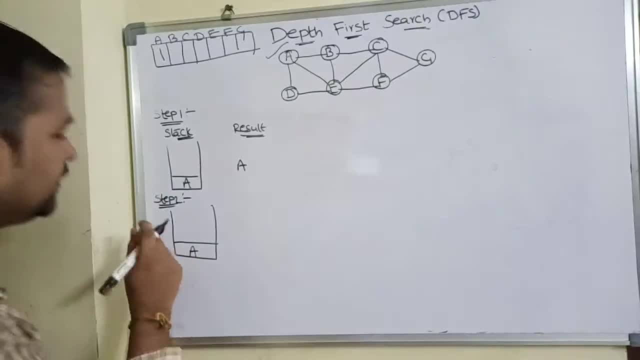 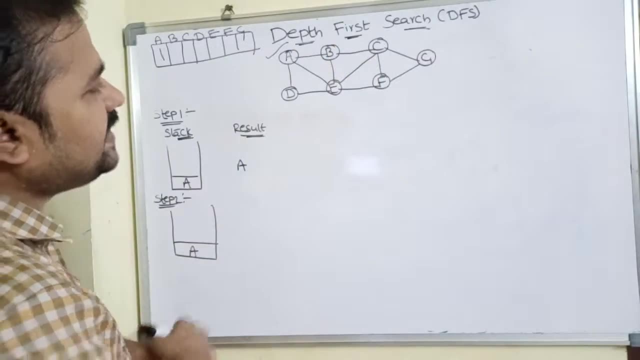 So here, initially, we have A on that stack. Next, what are the vertices adjacent vertices of A? We have B, D as well as E, but let us assume that this is level 0, this is level 1.. So 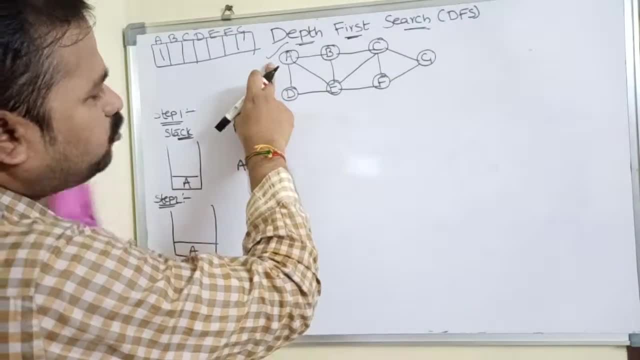 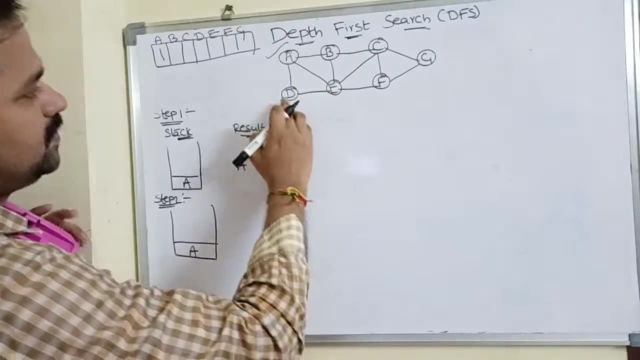 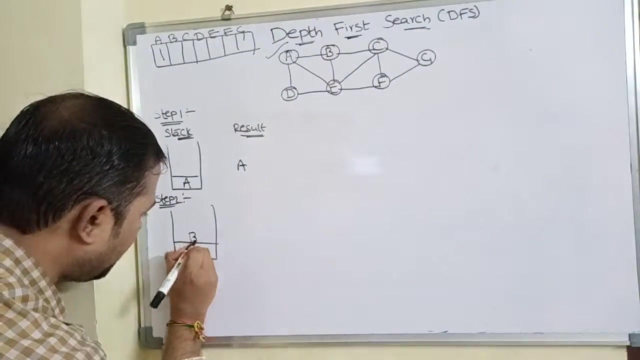 depth first search means starting from the starting vertex. we have to go till we get the deepest level. So it is better to select B here, other than D and E. it is better to select B because this is nothing but one level. So push B onto the top of the stack, So result is A. 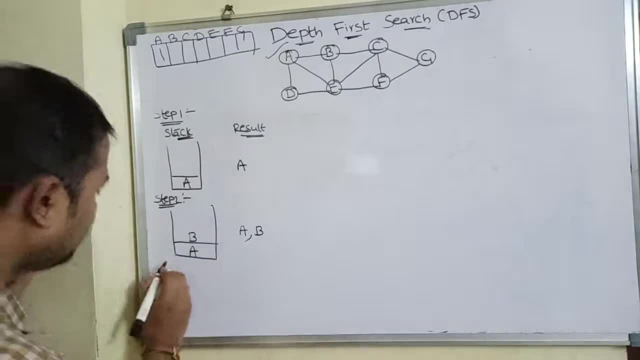 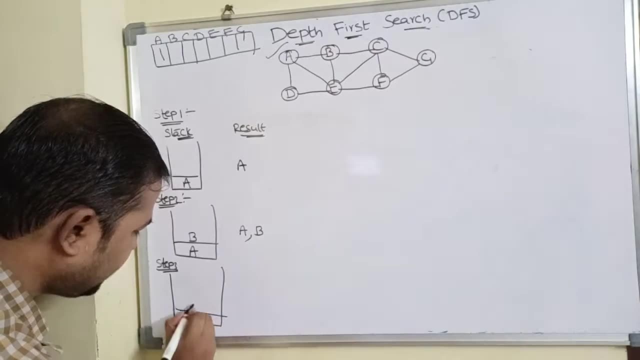 as well as now B is visited. so A, comma, B. Now let us write the next step, step 3, same process. While the stack is not empty, then select one of the unvisited adjacent vertex of B. Why? Because now the stack is not empty. So let us write the next step, step 3, same: 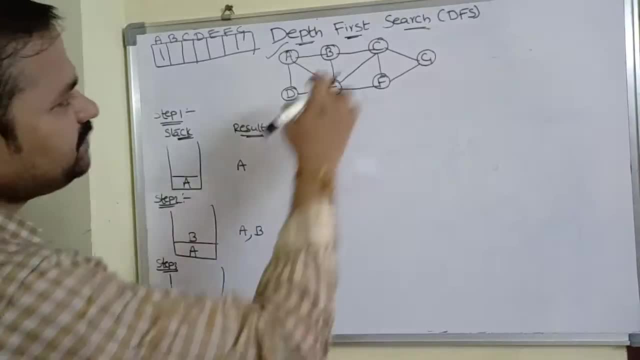 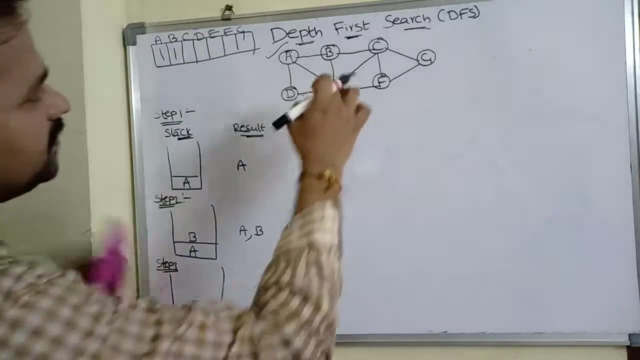 process While the stack is not empty. then select one of the unvisited adjacent vertex of B. So what are the adjacent vertices of B, C, E and E Here? B is visited, so we have to make the status A as visited. So the adjacent vertices of B are A, C and E, but A is already. 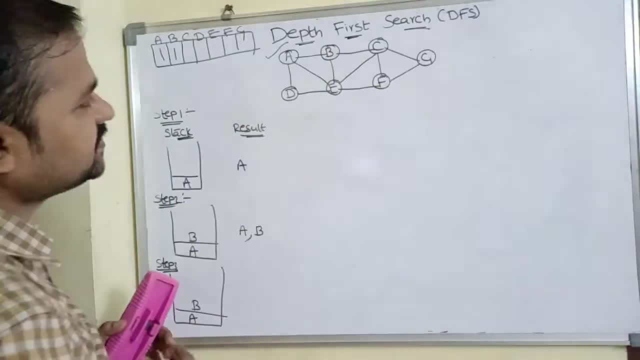 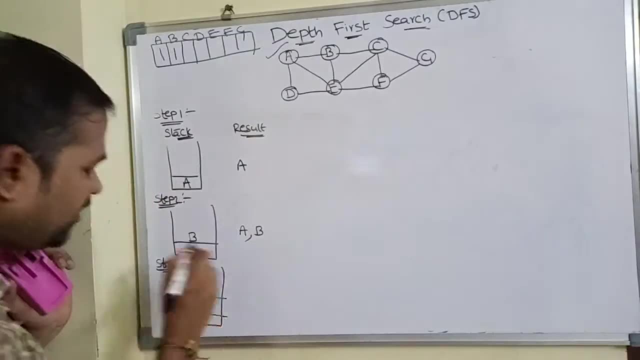 visited. Out of C and E we have to select one vertex, but it is better to select C here because this is nothing but one level. So select C and push it onto the top of the stack. So C is pushed onto the top of the stack. So we have to make the status A as visited. 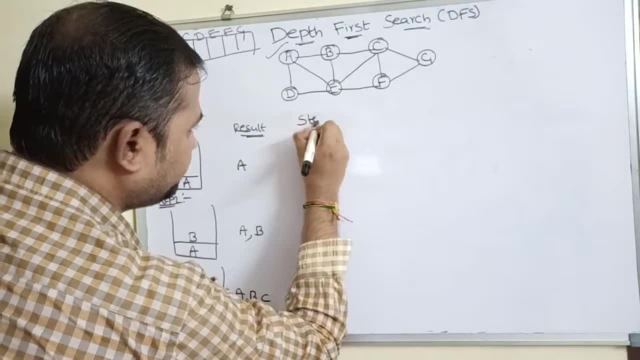 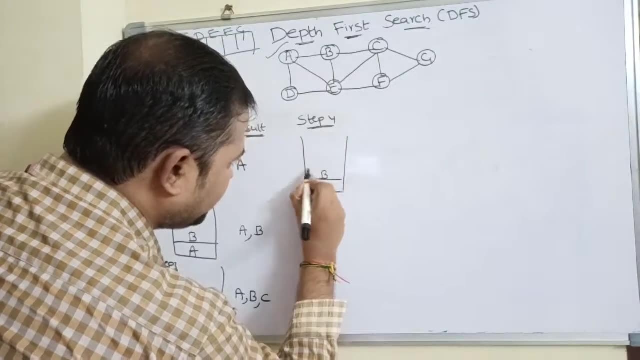 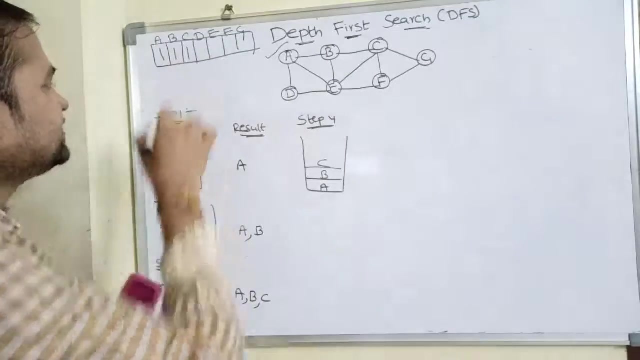 stack. so c is visited. now let us write the next step, step four, step four: a, b, c are visited. a, b, c are visited. and next let us take the adjacent vertices of a. here c is visited, so make the status as visited. so what are the adjacent vertices of c? because this c is at: 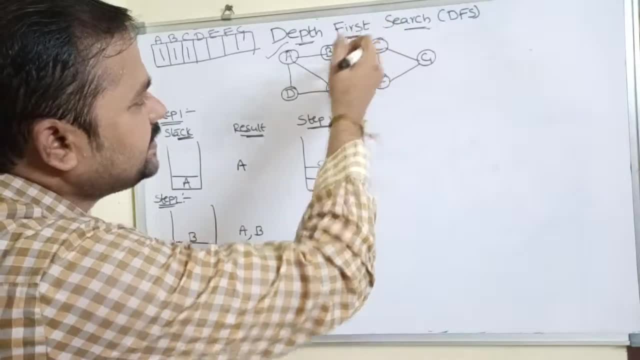 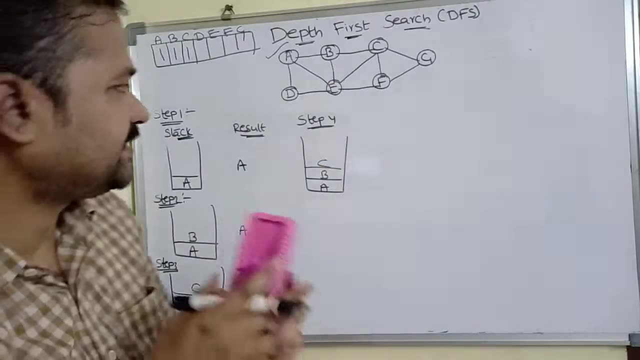 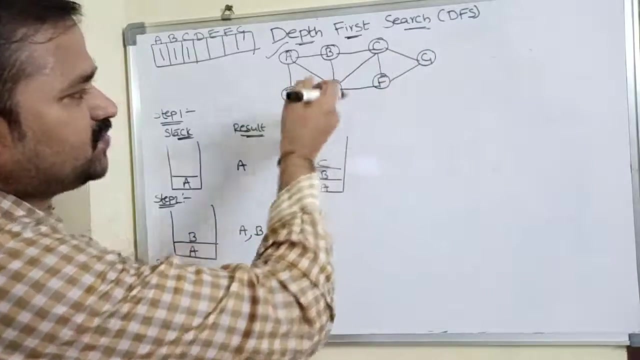 the top of the stack. so b, e, f, g, but b is already visited. so out of g, f, g, we have to select one vertex. but if we select g, then directly we can get the output. from g we can go to f, from f we can go to e, from e we can go to d. so there is no need of any backtracking. 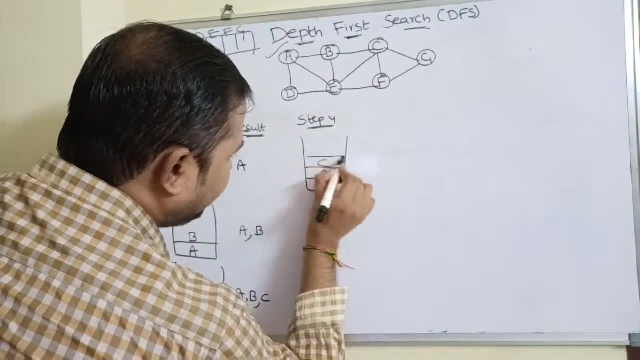 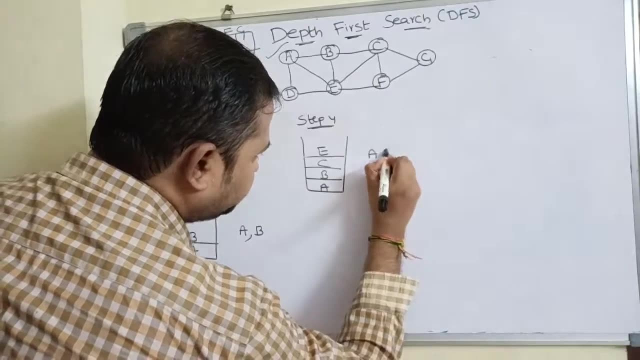 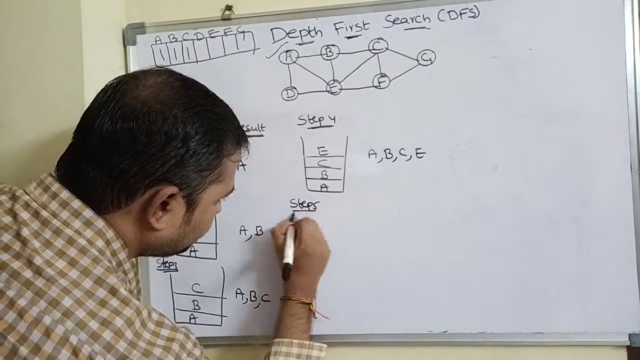 so that's why i'm selecting e here. so let us select the adjacent vertex e and push it onto the top of the stack. so previously the output is abc, now e is visited, so e will get into the output. next step, step five, step five. so what? what are the elements which are in the stack? 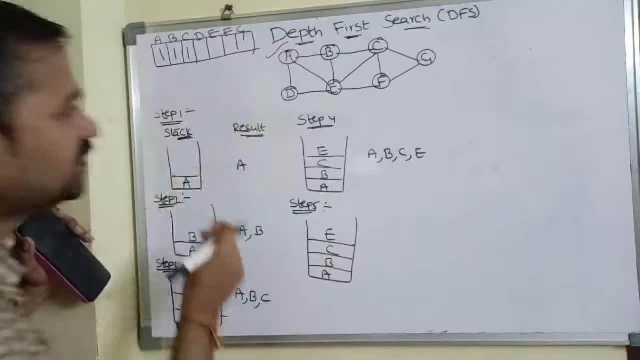 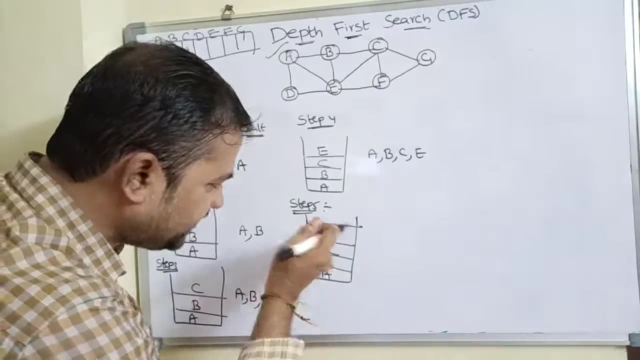 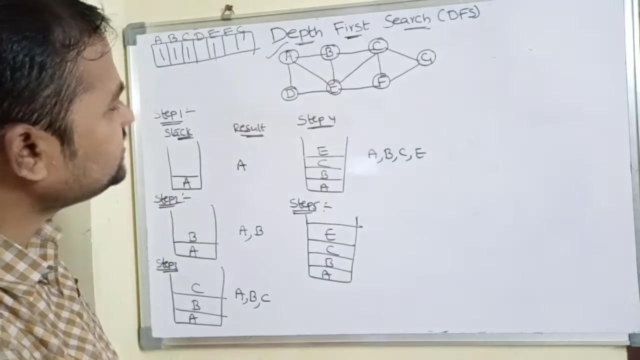 a, b, c, e, a, b, c and e. next, we, while the stack is not empty, here, the stack is not empty, so select one of the unvisited adjacent vertex of e. so what are the here? e is visited, so its value is one up. so what are the adjacent vertices of e? we have a, b, c, f and t. 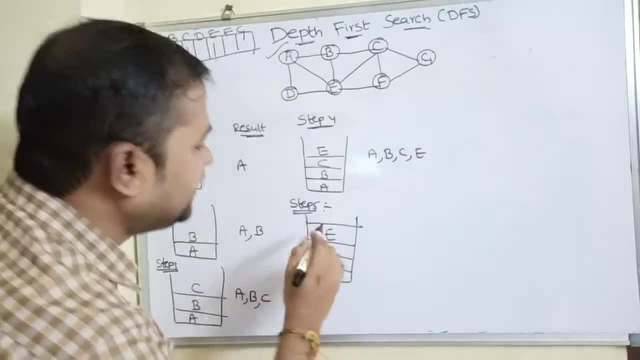 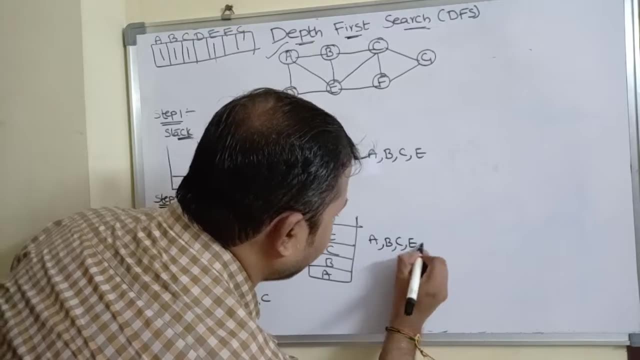 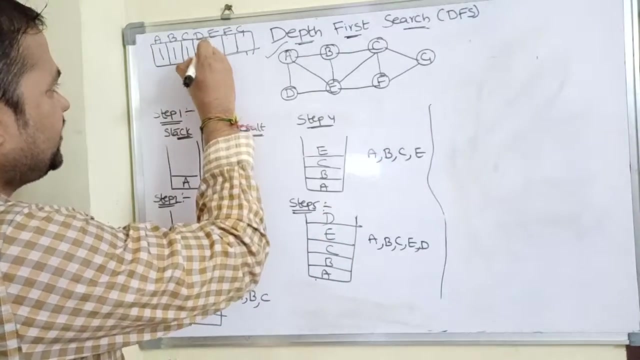 a, b, c are already visited. so here it is better to select enough, so d. so push it down to the top of the side and make the status as visited so a, b, c, e, d. okay next. so make the status of d as visited. so d has visited. so here we have one. so one specifies that t is visited. and now let us do: 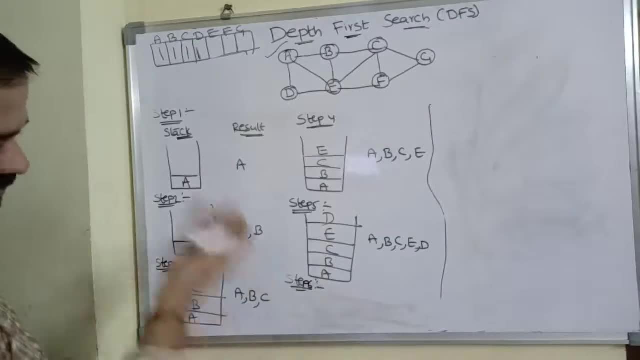 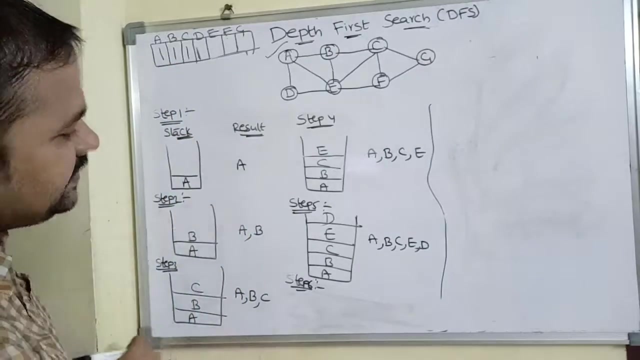 the next step, step six, while the stack is not empty. so here the stack is not empty, so we have to select one of the unvisited adjacent vertex of t. so what are the adjacent vertices of the a- e? but here a is already visited as well as e is already visited. okay, this e is already visited. 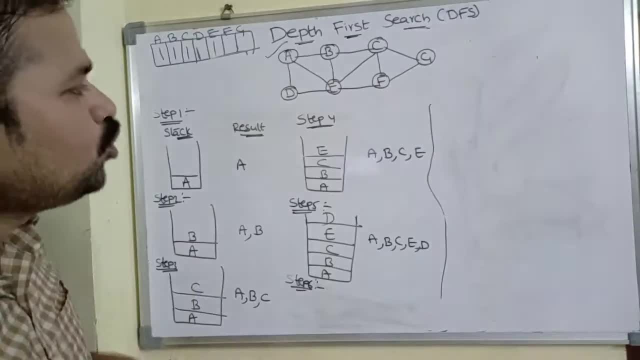 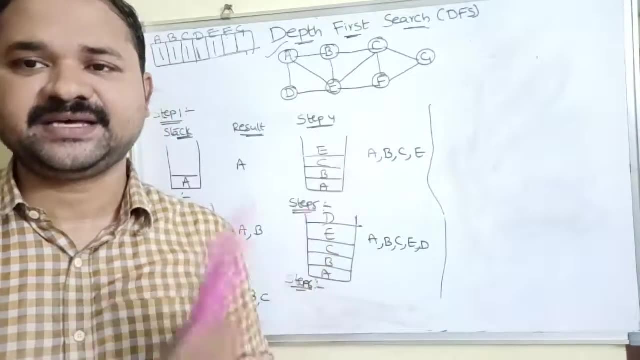 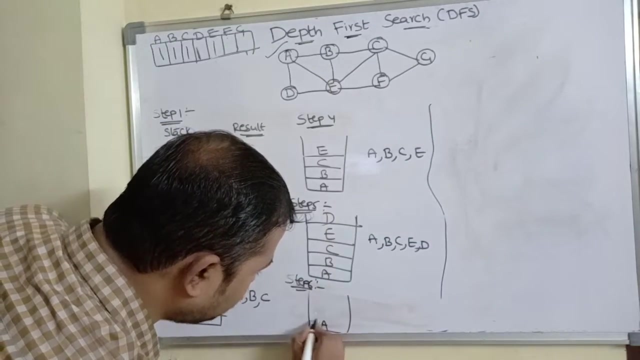 as well, as a is already visited, so there is no node to visit. so if there is no node to visit, we have to perform the backtracking. so backtrack means here a pop, an element from this stack. so what is the topmost element? d. so d will be powered from this stack. so the output here is: 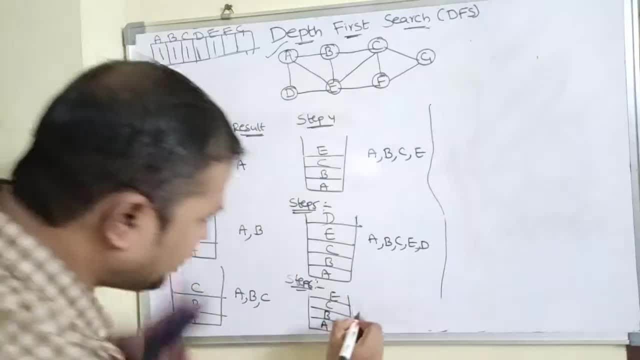 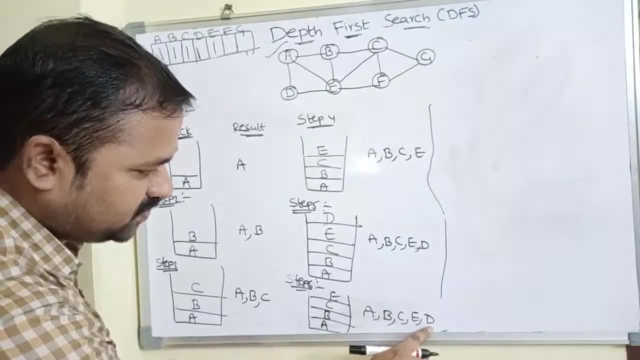 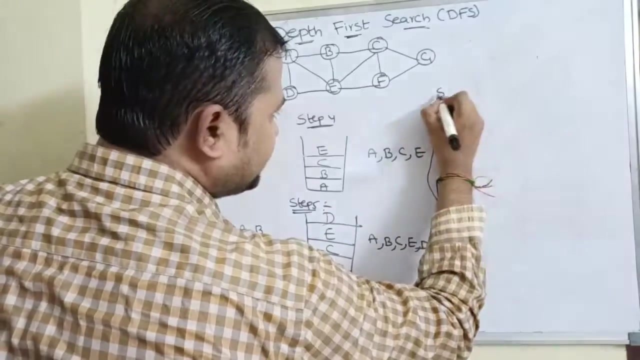 a, b, c, b. so this d will be powered from the stack. and here there is no change in the output. a, b, c, e, d. only here there is no need to delete. okay, only we have to delete d from this stack. only. okay, because we visited d, only d also okay. now let us do the next step. 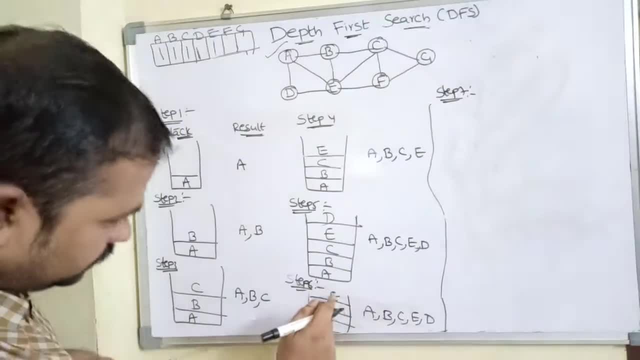 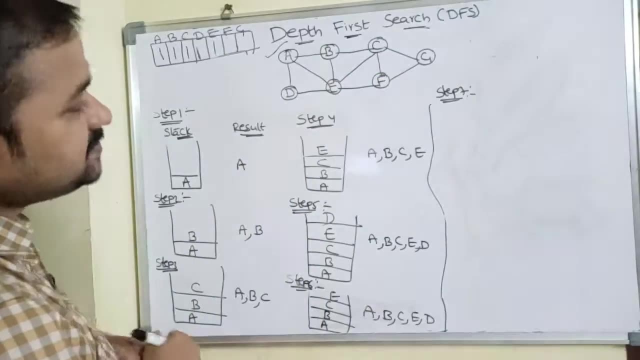 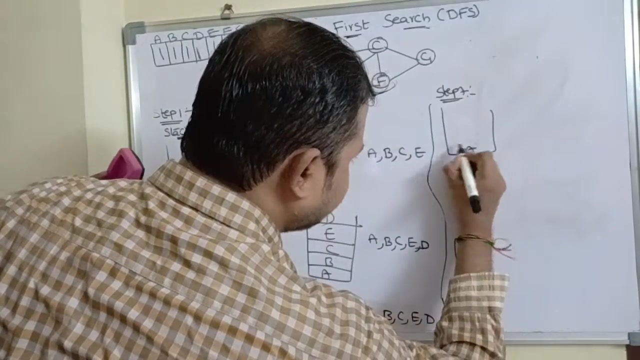 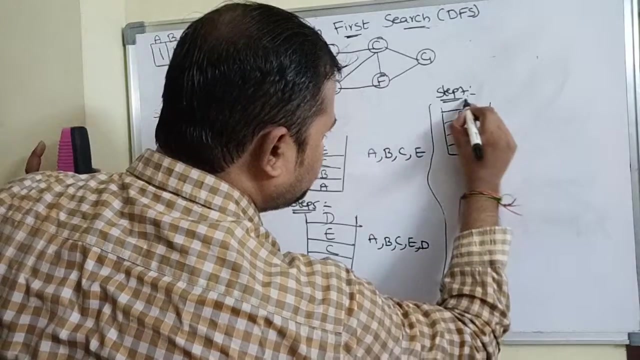 step 7. now we are at which node, e node. so what are the adjacent vertices of e, b, c, f? but b, c are already visited. f is not visited, so push f onto the top of the stack. so now the stack contains a, b, c, e. now we have selected f, so push f onto the top of the stack and mark the status as visited. 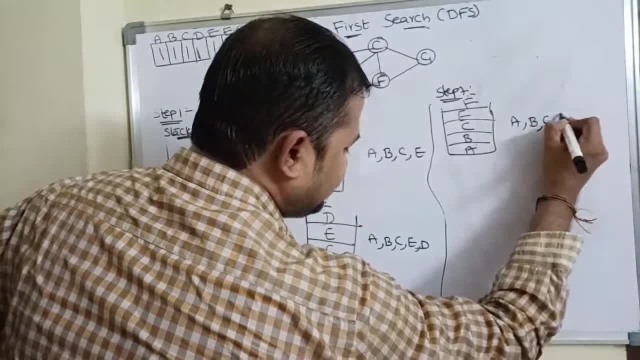 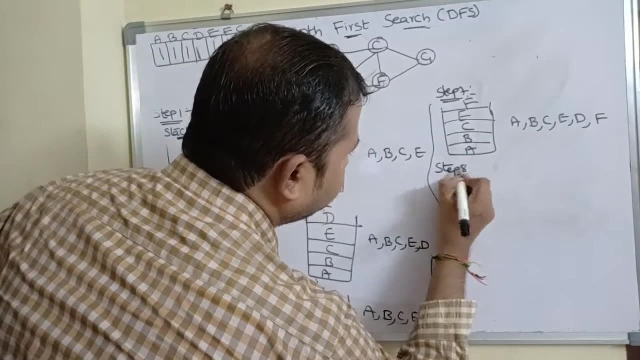 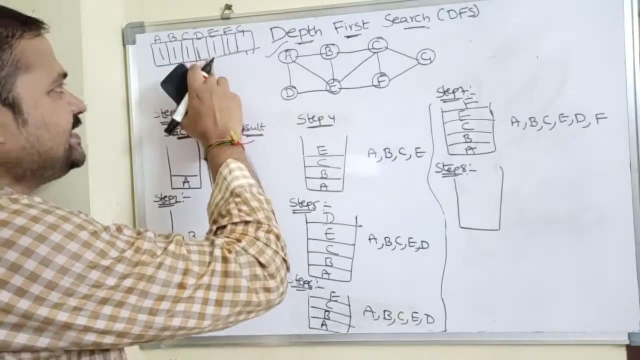 so what is the output now? so previously we have a, b, c, e, d. now we visited f, so f. now let us write the next step, step 8. so what are the adjacent vertices of f, c, e, g? but c is already visited, e is already visited, but g is. 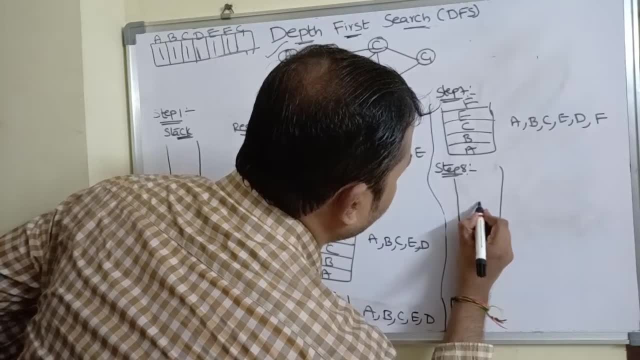 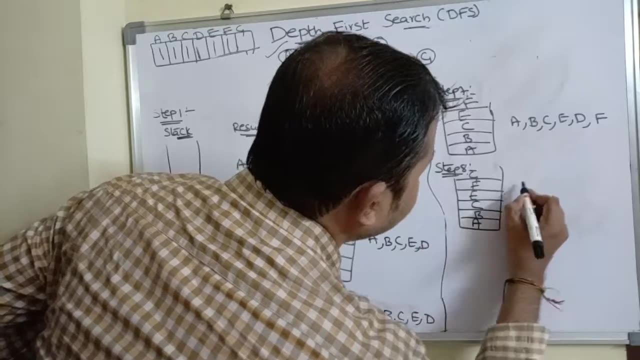 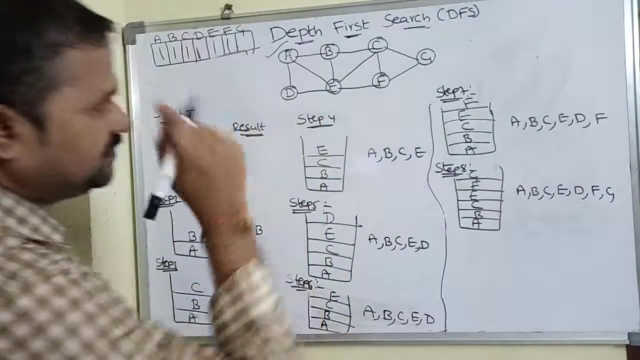 not visited, so it is better to push g onto the top of the stack. so a, b, c, e, f, g. okay, a, b, c, e, f, g. so now g is pushing. so the output here is a, b, c, e, d, f, g, g is pushing, so now we are at g now.